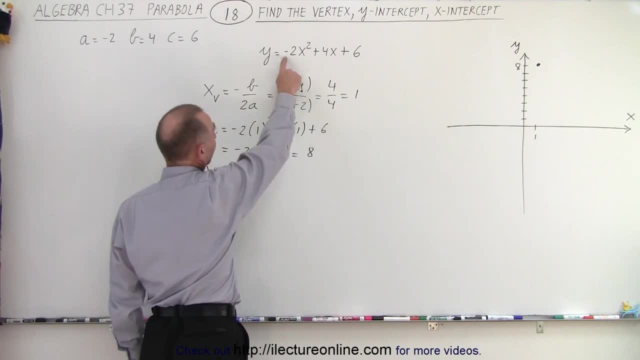 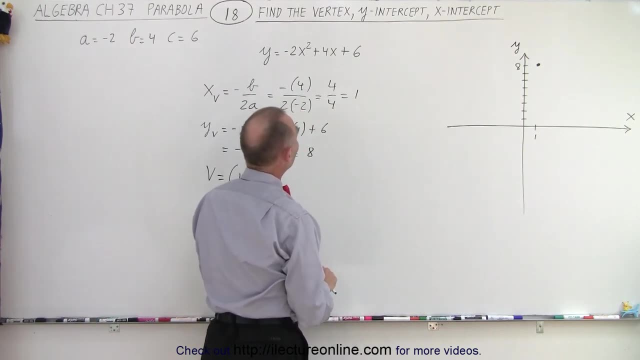 parabola starts. Next we realize that the parabola is going to open downward because we have a negative 2 in front of the x-square. So the parabola is going to go like this And next we're going to find what is easy to find, which is the y-intercept. The y-intercept is always going to 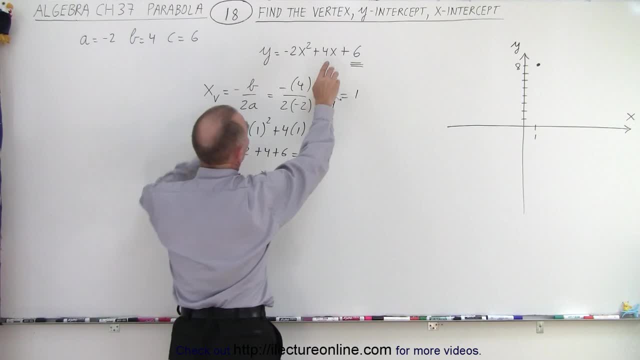 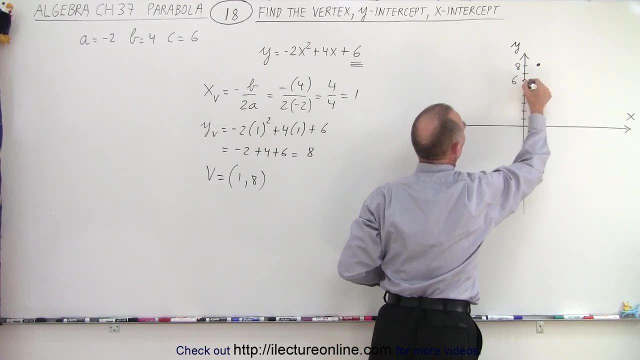 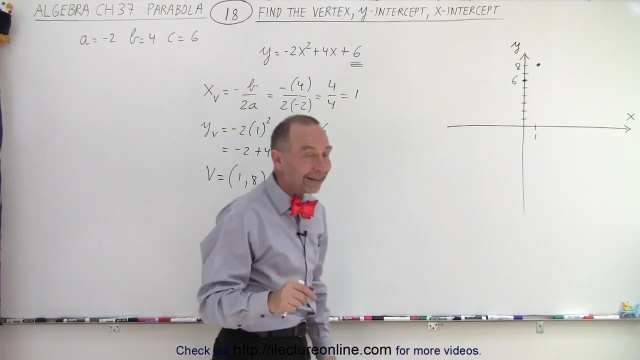 be equal to that constant at the end, because when x equals 0, this disappears and y equals 6.. So y equals 6. we know that the parabola will go to that point right there. And then you realize that, since the parabola is going to look like this, there's going to be two points on the x-axis. 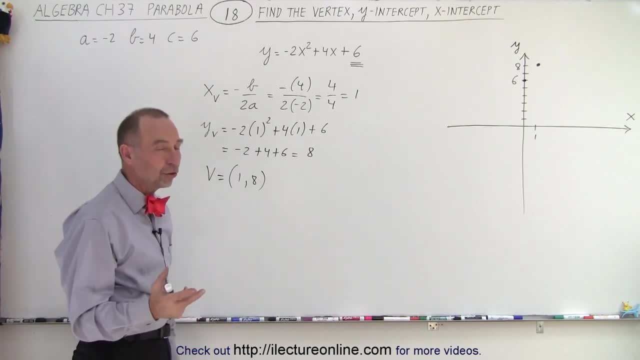 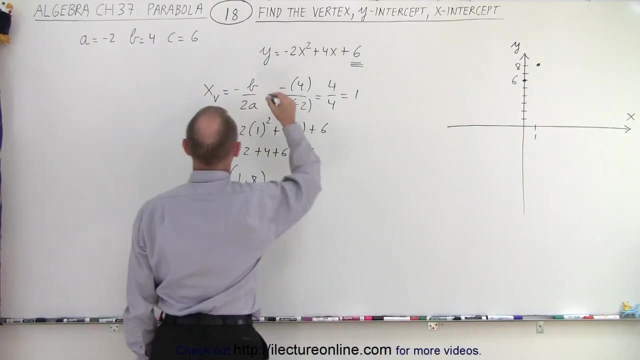 where the graph is going to cross. How do you find those two points? Well, you set y is equal to 0 because on the x-axis y is equal to 0. So to find the x-intercept, we're going to set y equal to 0, which means we end up with 0.. 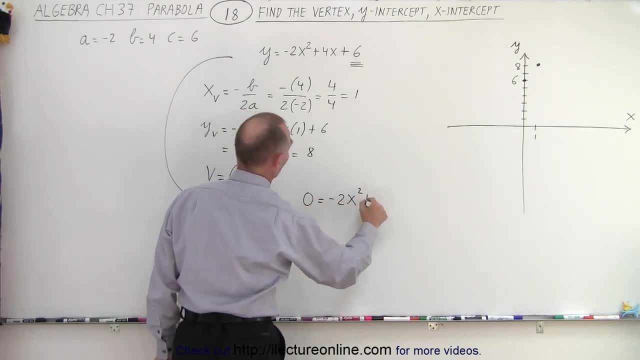 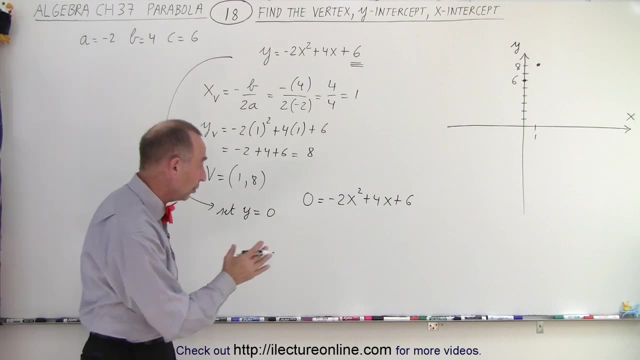 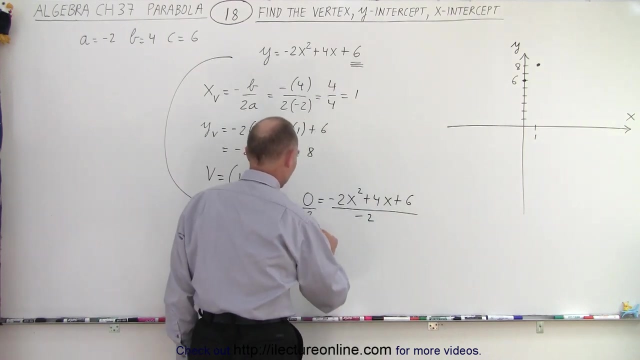 0 is equal to negative 2x squared plus 4x plus 6.. Well, the first thing to do when to make everything easier, is: we'll divide everything by negative 2.. So divide the left side by negative 2 and divide the right side by negative 2.. We get: 0 is equal to x squared minus 2x minus 3.. And now maybe that? 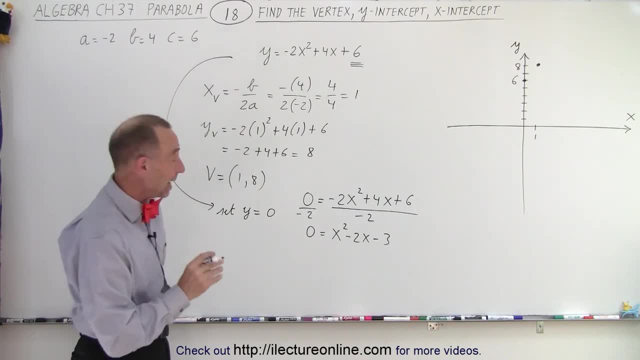 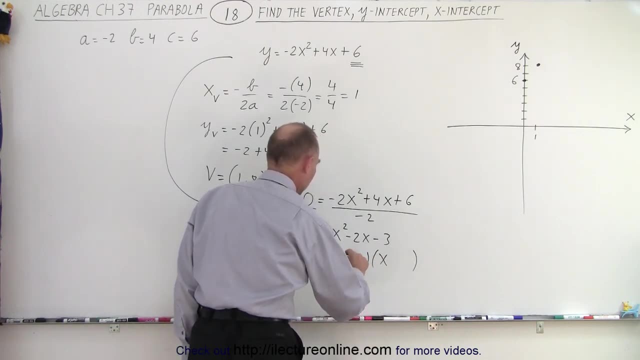 can be factored. Can that be factored Minus 3.. I think we can, So let's factor that. So 0 is equal to right. is the product of two binomials, x and x. We need a plus and a minus. How about a? 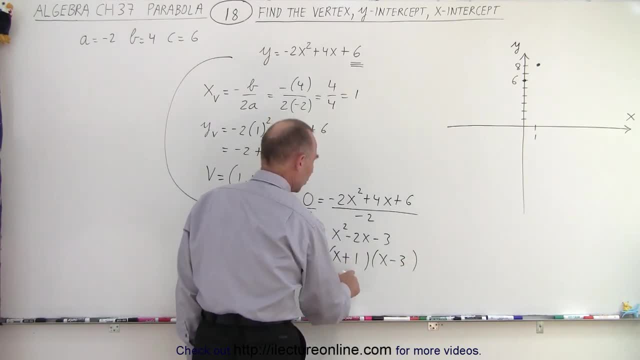 minus 3 and a plus 1.. When you add the two together, you get minus 2.. When you multiply, you get negative 3. Which means that x is equal to. Oh, let me, let me do it the right way. I was going to do a shortcut. 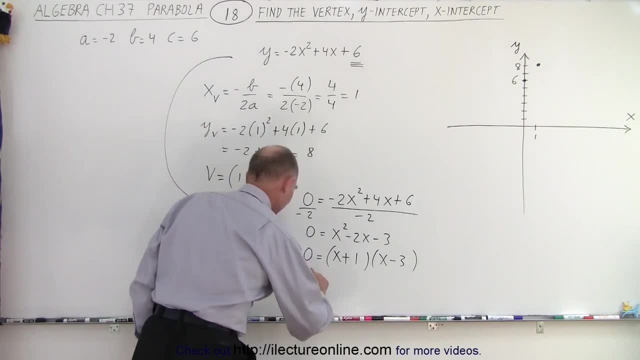 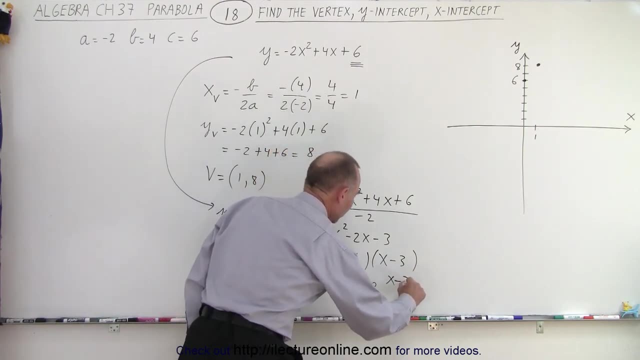 Never good to do shortcuts. So here we're going to say that x plus 1 equals 0, or x equals negative 1, or x minus 3 equals 0, or x is equal to 3.. So at those two locations on the x-axis, that's where the 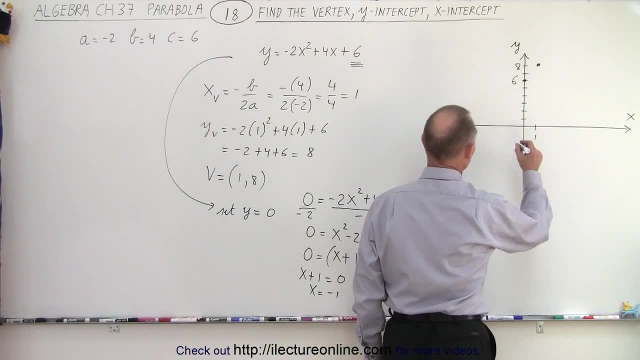 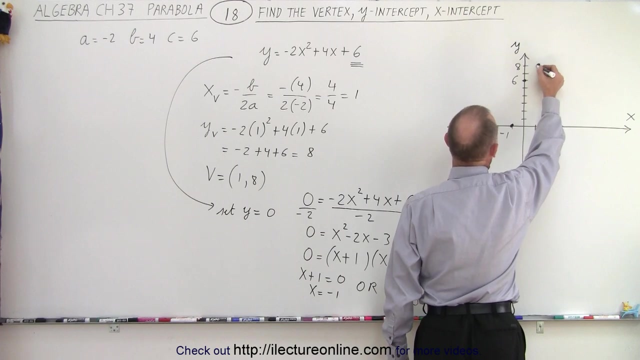 parabola will cross the, the x-axis. So x equals negative 1 and a positive 3.. So you know that the parabola will pass through here and through there. So now you have four solid points in order to help you grab the parabola, which makes a lot easier. So the first one will look like this, and on the 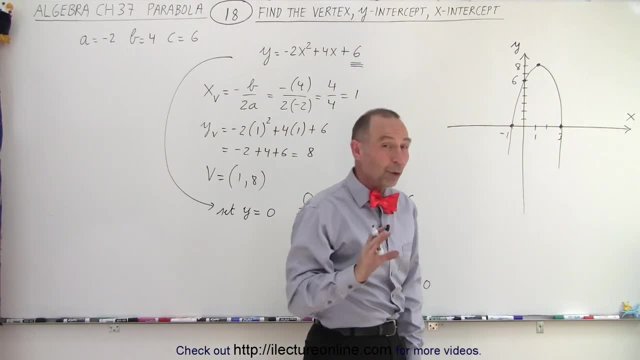 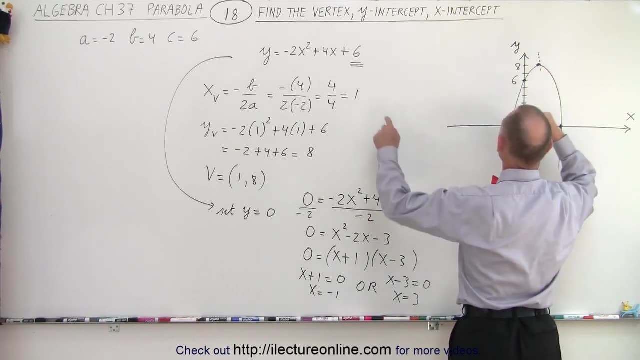 other side it'll look like this: I guess we could do one more thing, even though they didn't ask for it, Since we have an axis of symmetry, and that will be at x equals 1.. Let me try this again. There we go: x equals 1, like that, There's 1.. 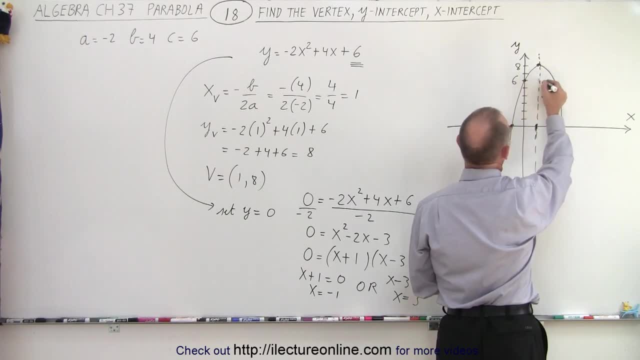 Okay, so we know that we had at y equals 6, we're 1 to the left of the axis of symmetry, So we go to the right one unit. This would be where we have. I guess that would be the point number 2.. That's. 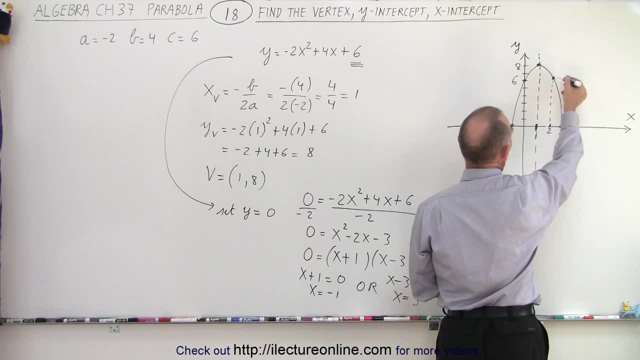 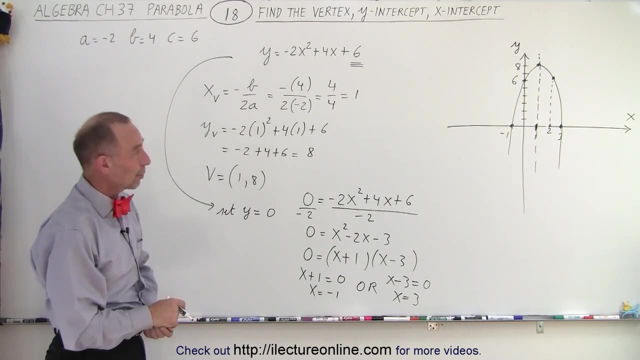 where we have another point Where we know we're going to go through. So this is also based upon the symmetry, about the axis of symmetry, where we can find another point to help us graph that parabola. And that is how it's done. 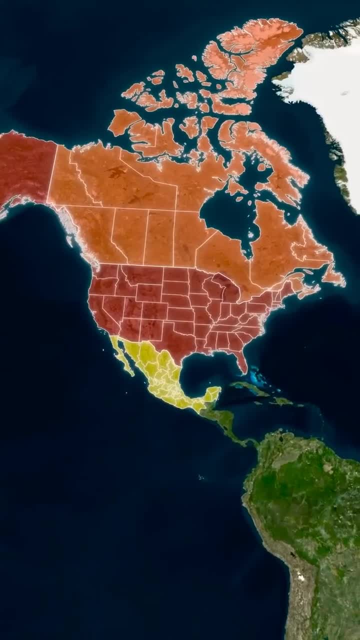 What is the largest country subdivision in the world? By this I mean what is the largest state, province or region of any country in the entire world? You might be quick to think of the US state of Alaska as the biggest, as it's the largest state in the US, but I was surprised to learn. 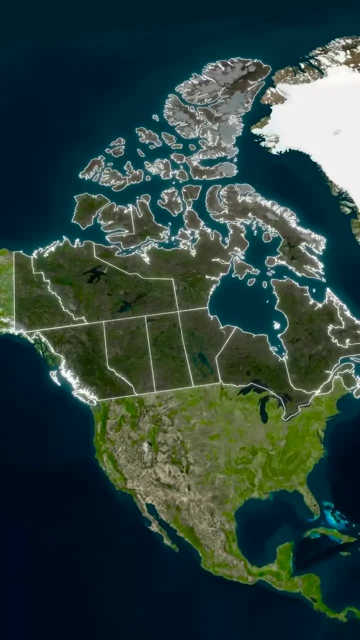 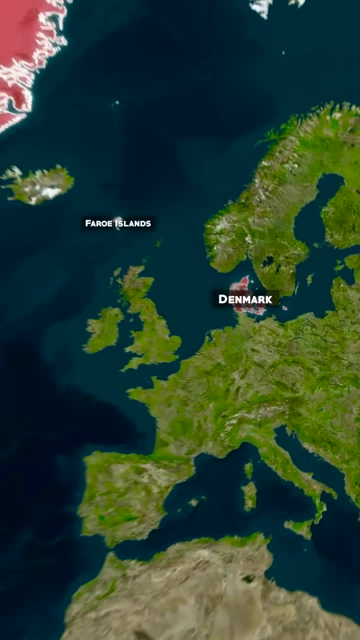 that Alaska is only the seventh biggest in the world, and Canada is the territory of Nunavut, a huge piece of land which is larger than the entire country of Mexico. The Kingdom of Denmark owns the island of Greenland, although it's debatable whether or not this counts as a single. 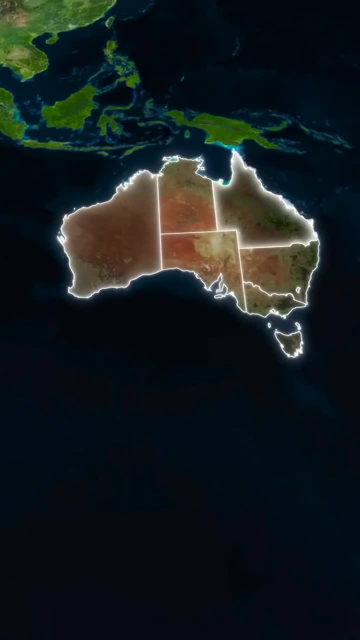 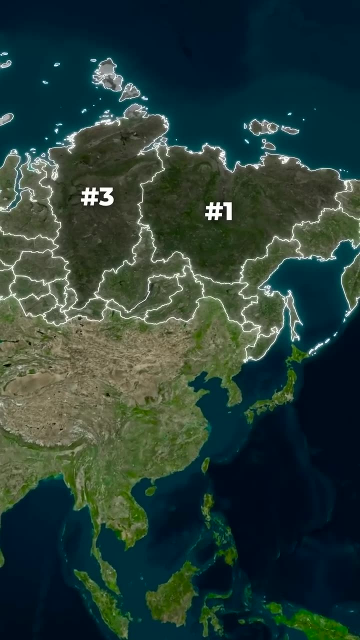 subdivision Over on the other side of the world. Australia owns two states on this list, which are Queensland and Western Australia. However, Russia owns two massive regions on this list which place at number three and number one, and these are the Krasnoyarsk Krai. 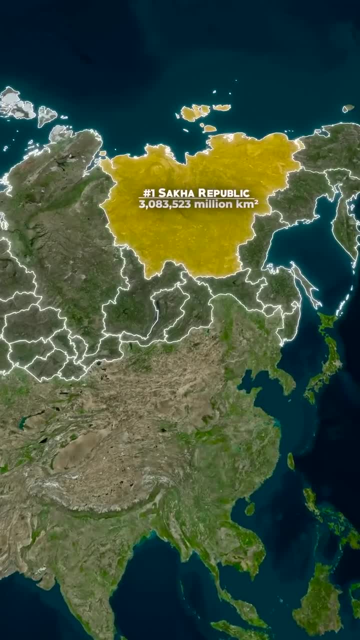 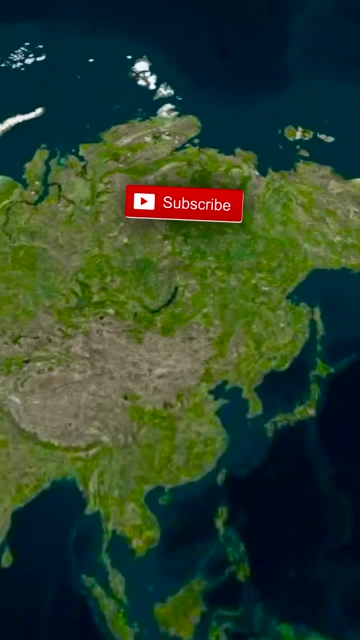 and the Sakha Republic. If the Sakha Republic was an independent country, it would rank as the eighth largest country in the world, larger than countries like Argentina and Algeria. Anyways, if you learned something, make sure to hit that red button. 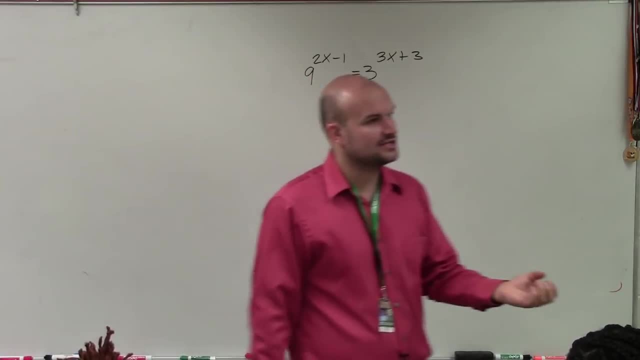 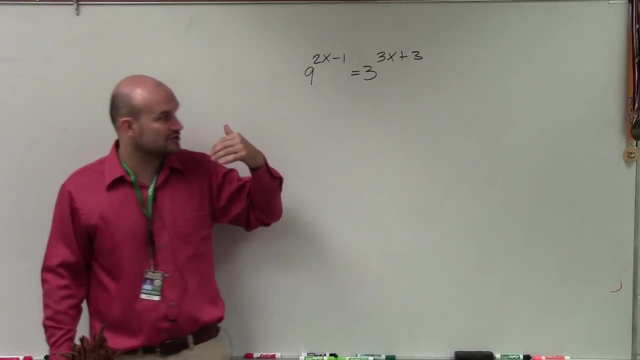 can't solve for a variable when it's in the denominator. So the best thing we want to do is we have to get the variable out of that power, And we'll do more of this once we get into logarithms and exponential functions. But this is again just a reminder, kind of a refresher.